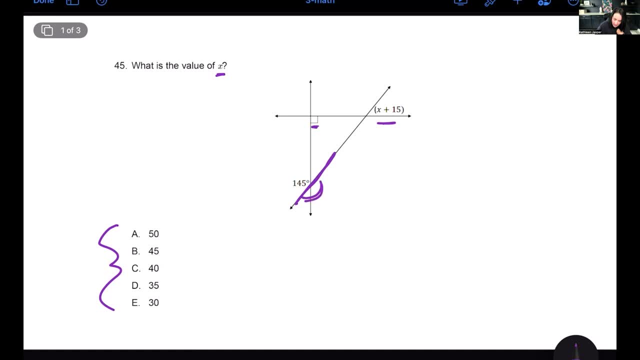 line here. okay, Okay, supplementary angles added up equal 180 degrees, because a straight line equals 180 degrees. So if I were to take 180 and subtract 145, I could find the answer to that little angle right there, because I need it in order to be able to figure out what x is in this situation. 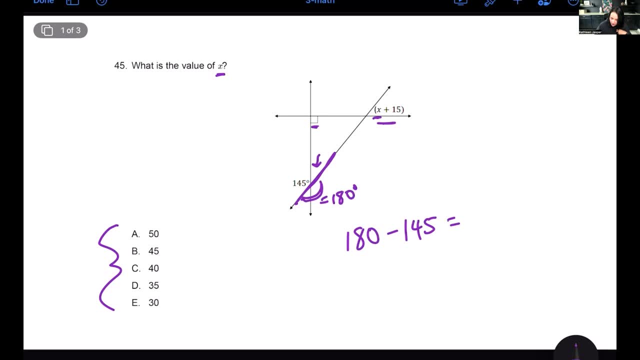 So 180 minus 145 is 35. So this angle- and let me just erase real quick because it's going to get messy- That angle, there is going to be 35 degrees. Hopefully you can read that, okay, Now I have a triangle. This right here now. 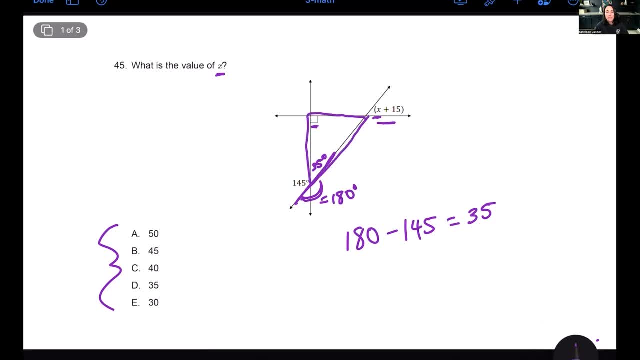 makes a triangle. So not only do I need to understand supplementary angles equal 180 and a straight line equals 180, now I can use what I know about triangles to figure out this angle here, And I'll just call it y for now, because I already used x in that parentheses up. 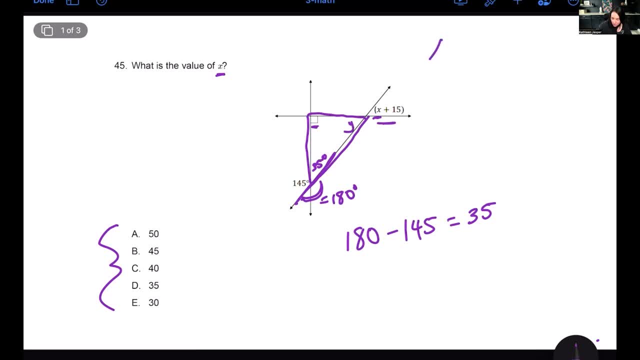 there. So let's try to figure out what y is. Well, guess what Triangles also equal 180 degrees. All right, So if I know, this box means that I have a 90 degree angles. Now, if you do not see the box, 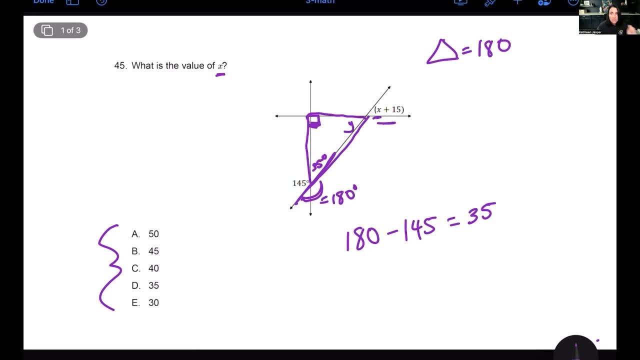 it is not 90 degrees, So be careful. Just because an angle looks like it's 90 degrees on the test, they will indicate it with that little box, So be careful. So right now I have 90 degrees plus 35 degrees plus y- I don't know what that is- equals 180.. 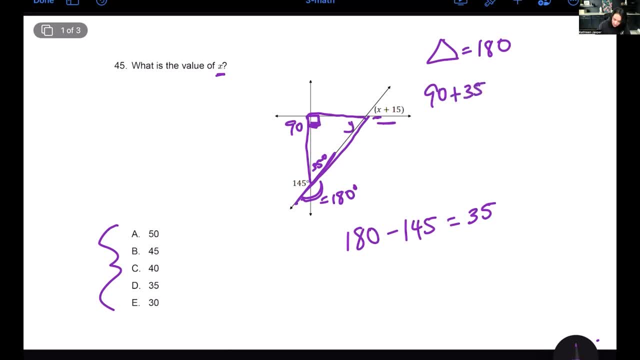 So 90 plus 35 plus this y- here we'll just call it y- equals 180.. So now all I need to do is take 90 plus 35 and I get 125 plus y equals 180.. So not only are we doing geometry here, 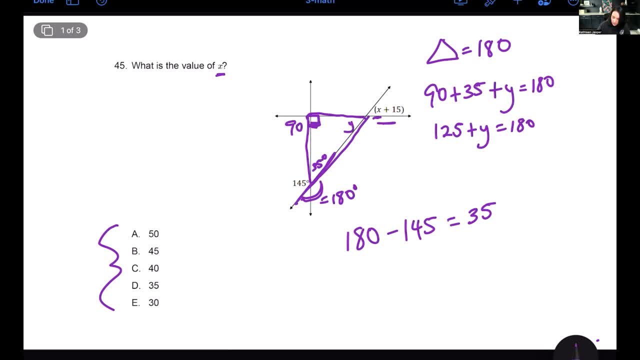 we're also doing algebra because we're going to solve for y. How do I do that? Well, I isolate this y here by subtracting 125, because that's a positive 125. And whatever I do to one side, I have to do to another. So I subtract 125. And in this case, 10 minus five is five. 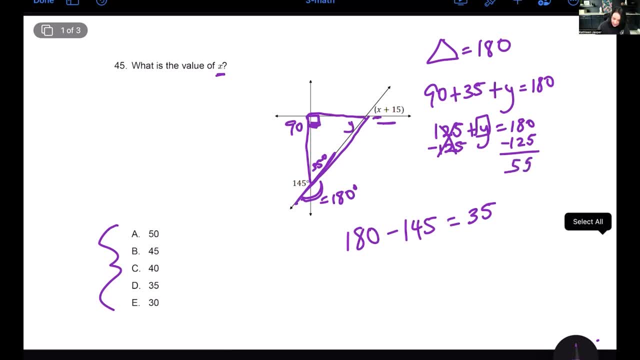 and seven minus two is five, In this case, this angle here, and let me erase, because now we know that angle, there is now 55 degrees, because 55 plus 35 plus 90. And let me just check my math, I got my calculator here: 90 plus 55 plus 35 equals 180.. All right, So now I need to use my 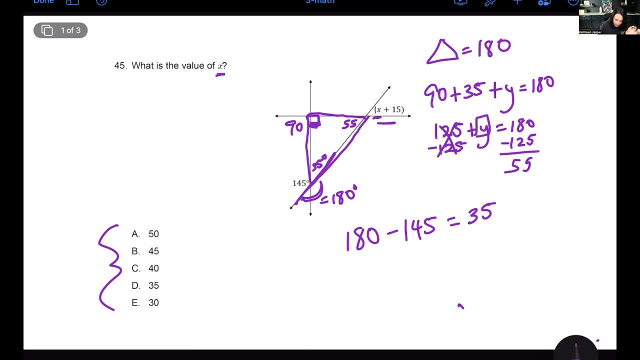 knowledge of vertical angles. So when you have- and let me just draw it here- these two angles are equal And these two angles are equal When they cross, at that point they're called vertical angles. So right here and right here are vertical angles and they are equal to each other. So in this case, 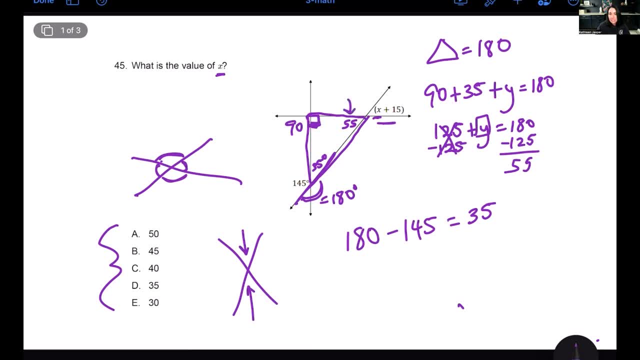 55 equals x plus 15.. So let me just erase a little bit more here so we can get some room. All right, So we have 55.. 55 equals its vertical angle, which is x plus 15.. Now let's solve for x again using algebra. 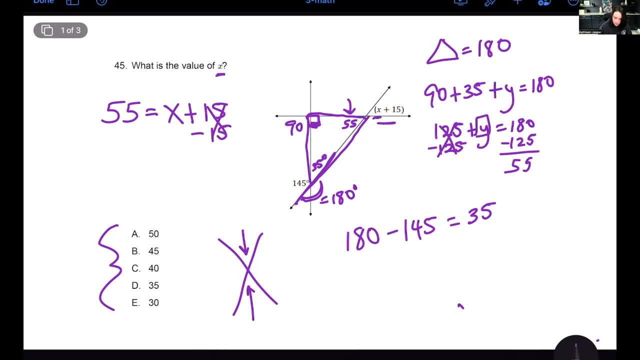 Subtract 15, because that's a positive 15.. So we do the opposite Subtract 15.. Five minus five is zero. Five minus one is 40.. 40 equals x. The answer is c. So notice, we did a few things here. 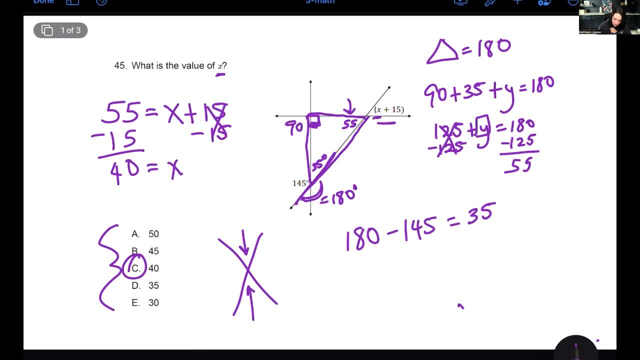 We figured out our supplementary angle. Then we got our promotion angle first, which was this: 35 degrees, because 145 plus 35 equals 180. We know that this line is a straight line here And supplementary angles together equal 180.. then I 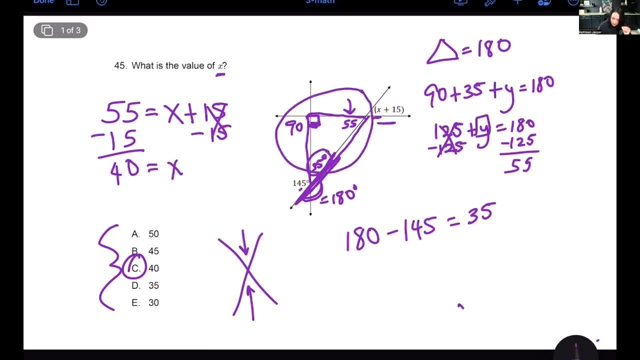 took a look at this triangle here and was able to find this particular angle here because I knew the box indicated 90. I had the 35 degrees from my previous Discovery: 145 plus 35 equals 180.. Then I had the discoveredballed base. The first union of this direct line is the 30. Now what I wanted to do was to find the diagonal of the Beach front. now again, I need to be able to record this chart. So I do that here, but you could do it here. but I can count on my self- UTILITIES pod and multiply that by malSen----ffil bulb. I try to get this in this problem. each time the point was to love your keg period, I had to modifyiana program here. 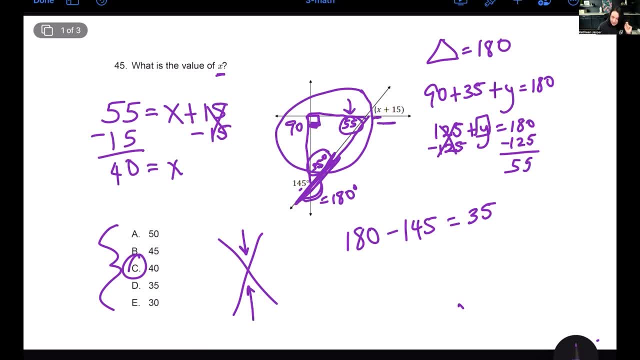 equals 180.. And now I know, if I add 35 plus 90 plus 55, I'm going to get that 180, which triangles all equal. all of the angles inside of a triangle equal 180. And then I have to use my 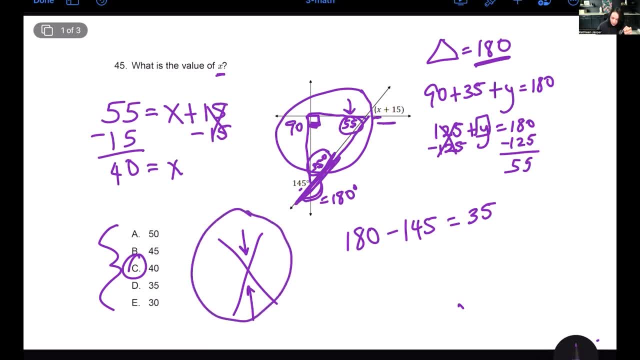 knowledge of vertical angles, like we did here, And we know that 55 in this case is going to equal x plus 15. We use algebra over here and we got our correct answer with x equals 40. So lots of skills going on in this, but just slow down and remember complementary supplementary rules of. 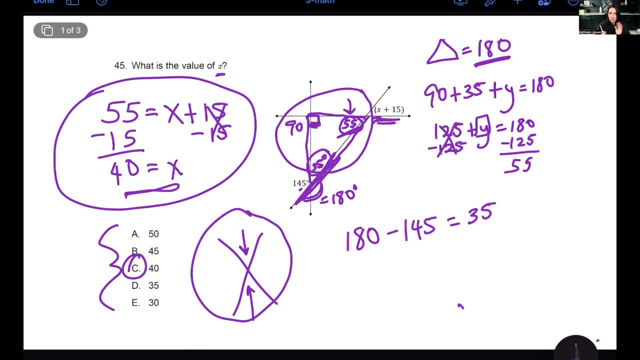 triangles, things like that. We cover them all in the book. we have charts that put them in a nice visual for you So you can check those out, And that is essential in solving a problem like this. All right, now let's go to the next question here. All right, So this is a word problem. 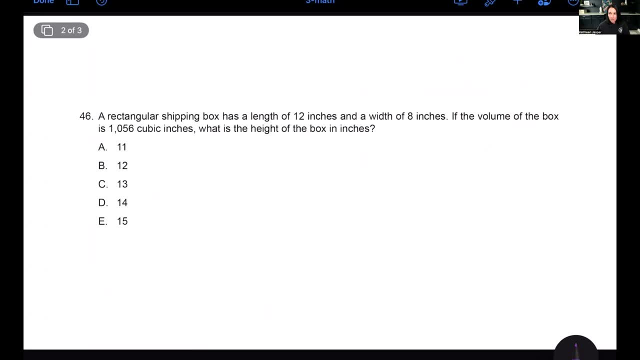 And a lot of people have trouble with word problems And it is a geometry problem. So I always like to start with my answer. choices can't do much here. They're just numbers. So let's have a look at the question. a rectangular shipping box? All right. as soon as I hear shipping box, I'm going to think volume. 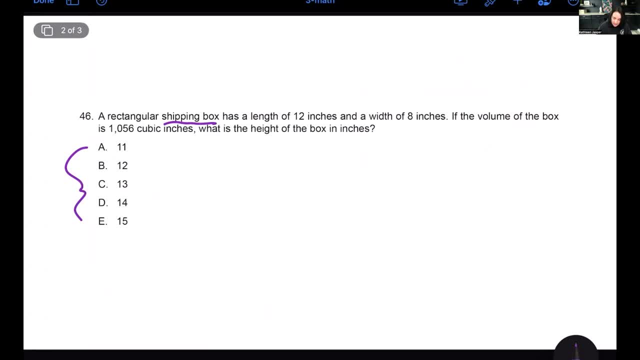 because I'm going to be putting stuff into the box. right, Has a length of 12 inches, So I've got a length of 12 and a width of eight inches. Okay, both of them are in inches. That's good news. I don't have to convert anything If the volume of the box is 1056 cubic inches. 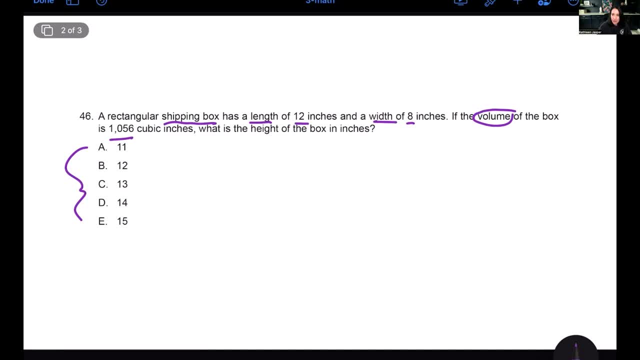 what is the height of the box? All right, and so you might be like: oh my god, how do I do this? This is very simple. We're talking about volume here. volume equals length times width times height. That's why they call it cubic inches. because it's going to look like this, Because you 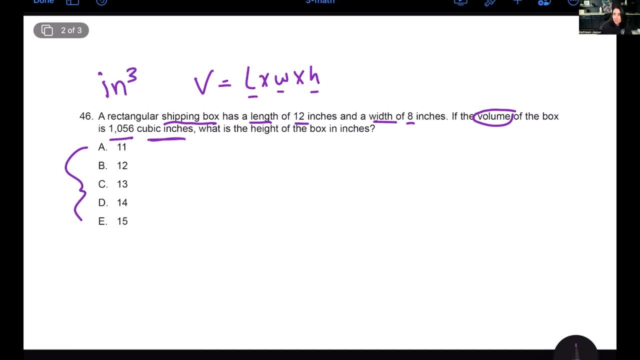 have three measures here: length, width and height, because it's a three dimensional figure. Now, all we do is use this formula in order to solve the problem. Well, I have the volume right. I have this V here. this V here, it's 1056.. See 1000, the volume of the box is 1056.. So I just hit equals. 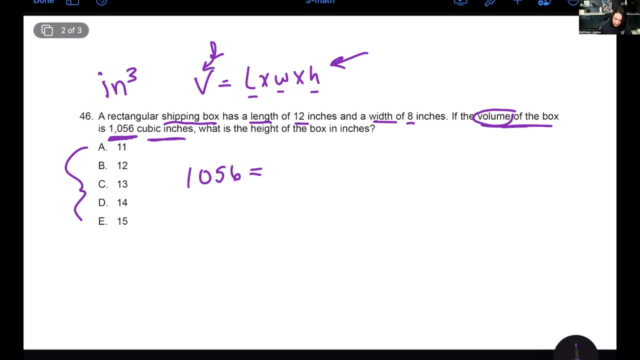 I'm using the formula And I have the length. the length is 12.. So 12.. I'm just going to put these in parentheses here to keep them organized. And I have the width, which is here eight inches eight, but I do not have the height. The height is unknown, but I have everything else, so I can. 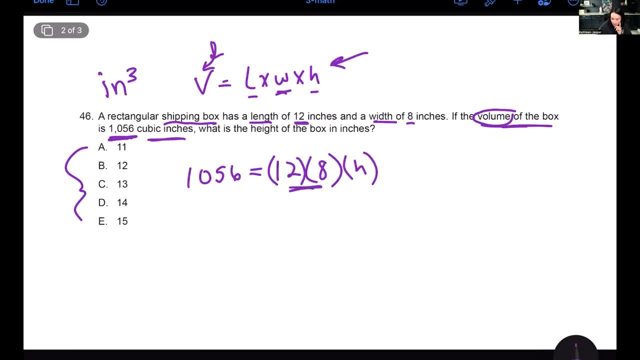 figure it out. So all I'm going to do is I'm going to multiply 12 times eight and I get 96.. Don't forget this H here. that is multiplied by everything. So this becomes 96. H equals 1056.. And then you can use your calculator. 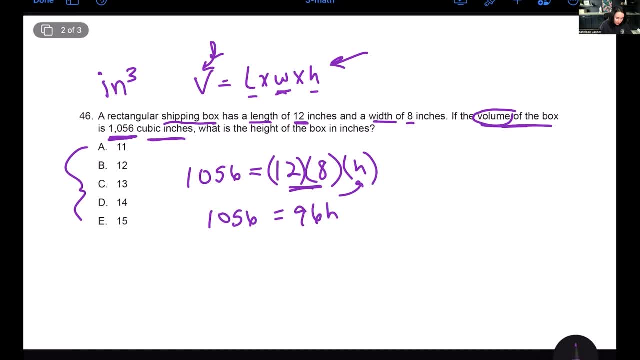 remember it will be an on screen simple calculator. be careful with it. 1056.. And we're going to divide both sides by 96 to solve for H, right, Because the 96 is attached to the height, we need the height to be isolated on its own. If we're multiplying 96 by H, we're. 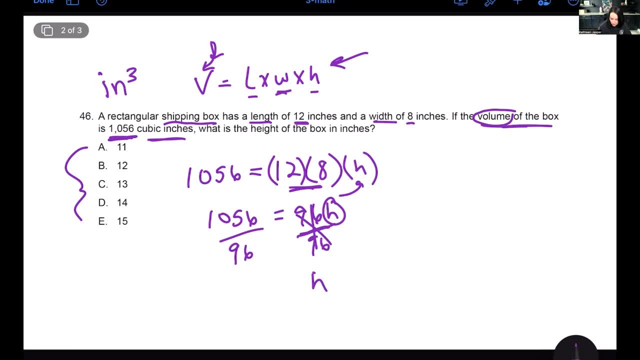 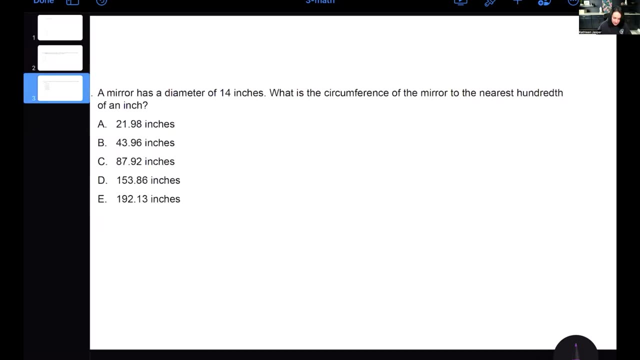 going to divide and that cancels, leaving us with just the H. what I do to one side, I need to do to the other, And that becomes 11.. H equals 11. answer a: All right, Now let's take a look at the last one here. And a lot of people. 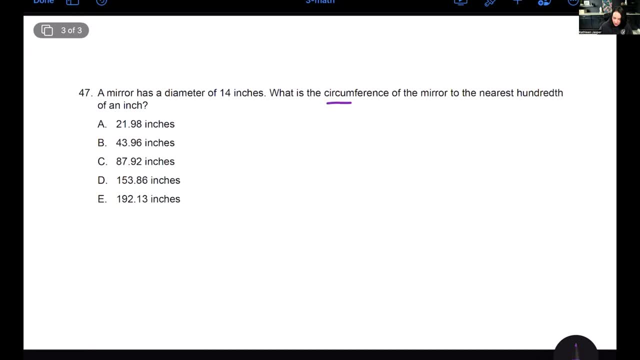 get freaked out about this, Because we're talking about circumference. I can see diameter, circumference and I'm like, Oh my god, it's a circle. It's a circle, It's okay. One of the things we want to see here is: I always want to look at my answer choices because it is going to give me a hint. 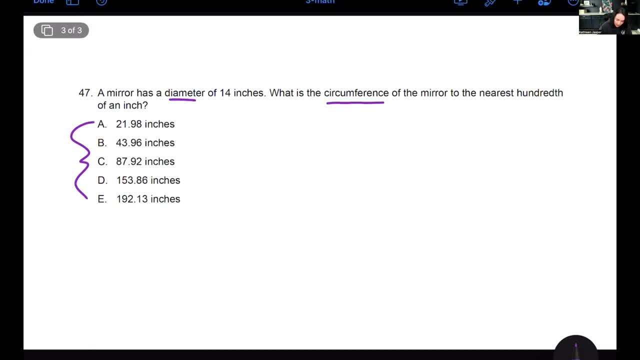 Notice that the answers are not in pi. these numbers aren't like 21.98 pi, So in this case we're probably going to have to figure out the pi by multiplying by 3.14.. It'll be clear in a second. Alright, so I have a mirror. has a diameter. 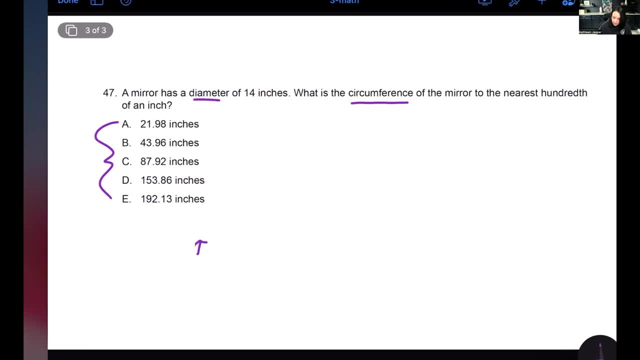 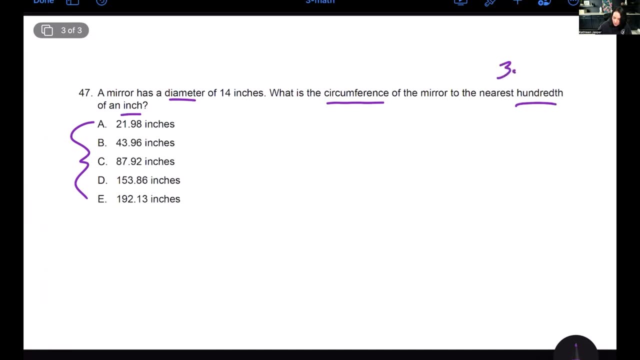 of 14 inches. What is the circumference of the mirror to the nearest hundredth of an inch? All right, They do that hundredth of an inch because we're going to be using 3.14 for pi And notice that the four is at the hundredth. 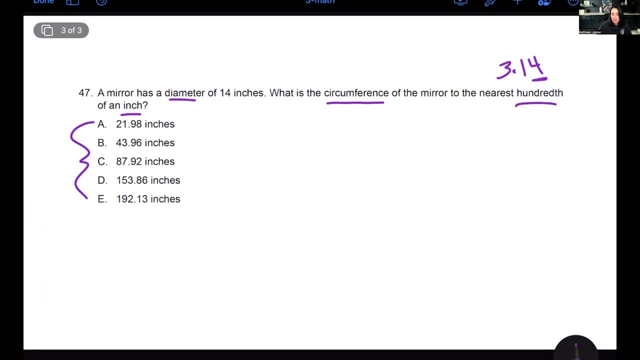 And it means basically that you can just multiply by 3.14 and not the entire number of pi, which goes on into infinity for all of my math nerds. So let's take a look. First I'm going to draw the circle. 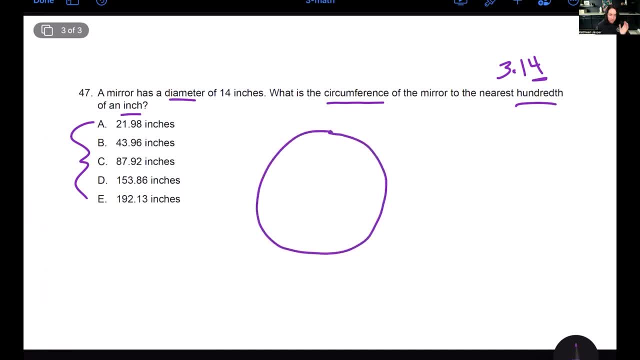 I'm gonna do my best. That is not a very good circle, but it'll have to do. Now, the diameter is the line that runs directly through the center of the circle right. So here's: the center runs directly through the center And the diameter is 14 inches. 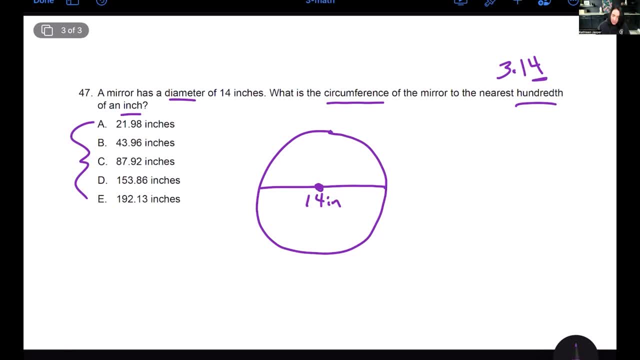 Now be careful that you understand the difference between radius and diameter. Diameter is the entire line that goes through. radius is from the center of the circle out, So that's the radius there. Let's use the formula for circumference. So circumference equals two pi r. Now, I know this because I teach math all the time. you may be like 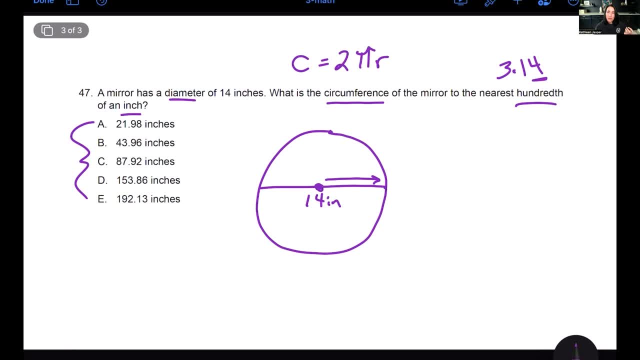 how did you find that you will get a formula sheet on the exam? it is available. it's usually an on screen formula. it's like a button: you click and the formula sheet comes up. At the end of this video, I'm going to show you what it looks like, based on the study companion. 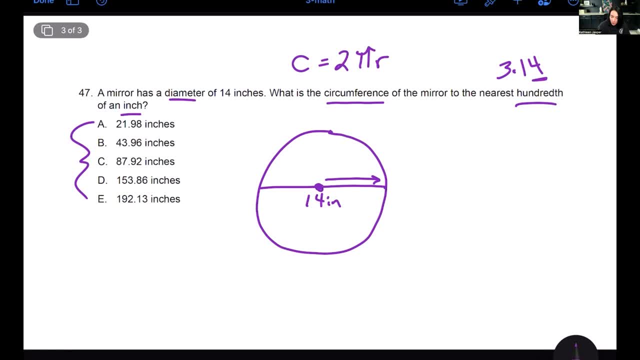 it's a very simple formula sheet, but you will be given this formula So I can look. now the circumference is what they're asking for. circumference equals two pi r. All right, Now, notice this pi here. That means I have to add in this 3.14., Because my answer choices are not in. 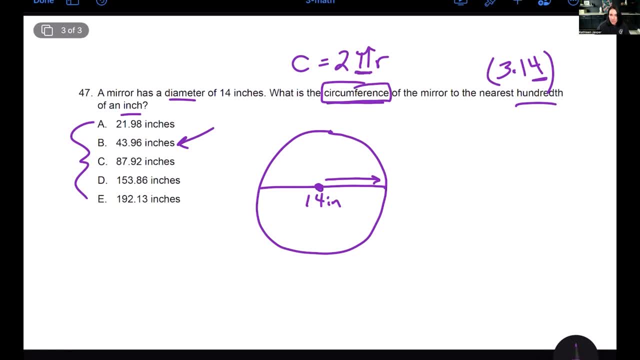 pi, so I have to actually multiply it by the 3.14.. So in this case, 14 inches is the diameter. Well, the diameter is twice the amount of the radius, right, Because the diameter is the full length And the radius is half of that. So what's half of 14, that's going to be seven inches, which. 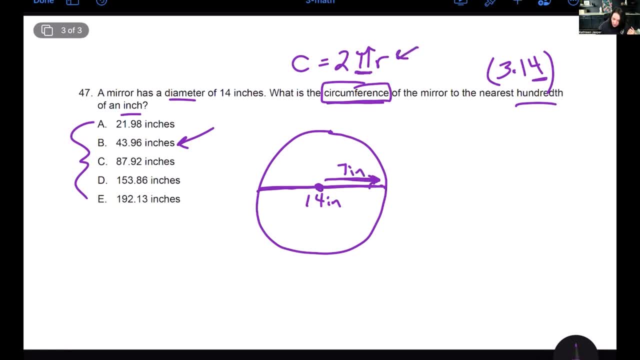 is important for our formula here. So we have: circumference equals two and this is pi. So I'm going to go ahead and do it 3.14 times r. Well, r, we know, is seven inches, We can just put them. 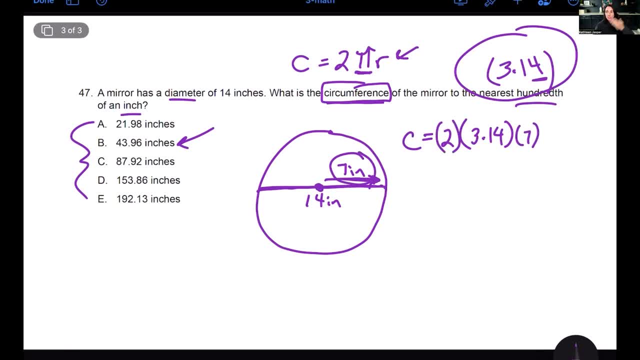 all in parentheses here to keep them organized right. So now we have multiplication on the right hand side. you can multiply these any way you want Because, remember, multiplication and addition can be done in different order, it doesn't matter. So let's just multiply the two by 3.14.. 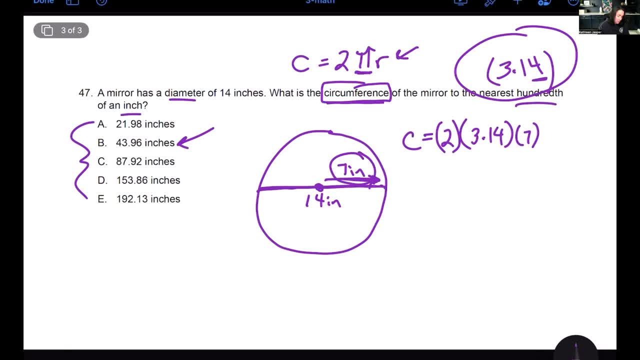 And we get 6.28.. And then multiply it again by seven and we get C equals 43.96.. All right, Now let's say we just want to kind of do this quickly And we don't want to be bogged down with the 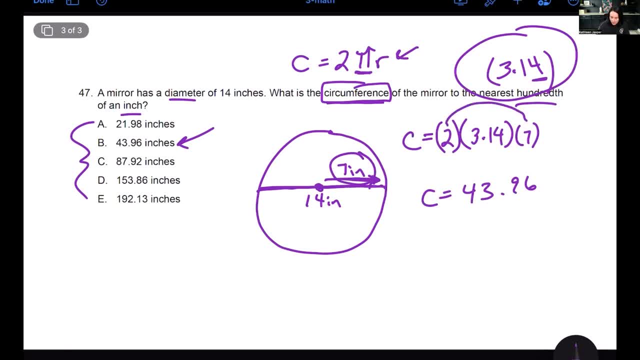 calculator. Okay, fine, Let's take two times seven, That's 14 times 3.14.. Let's say I want to just quickly look at my answer choices and see if I can eliminate. Well, let's say I want to just look at. 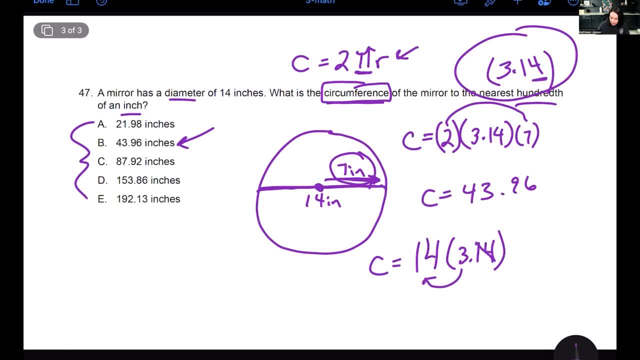 my answer choices and see if I can eliminate. Well, let's just multiply three. let's forget about the point one four here. Let's multiply three by 14.. And what do I approximately get here? I get approximately 42, right? Well, that eliminates a, that eliminates C. D is way too big and E is way. 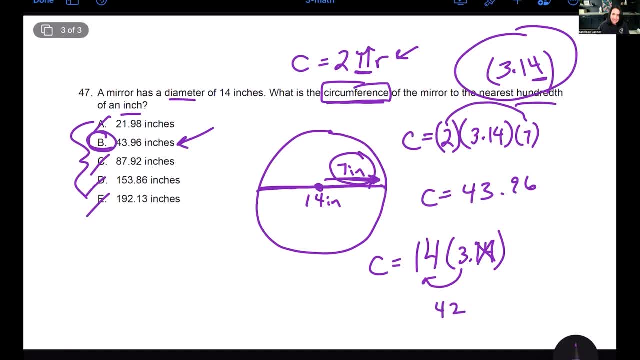 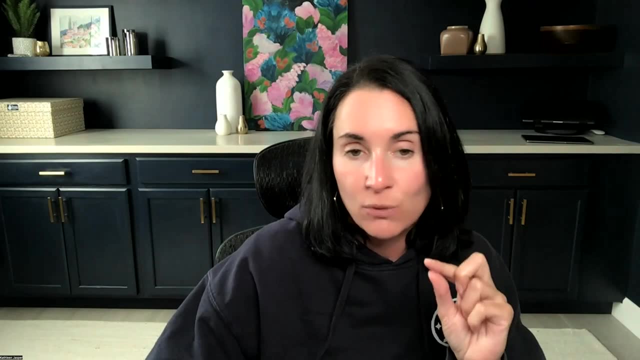 way too big, which leaves me with 43.96 inches. And if I were to multiply that 14 times 3.14, which is pi, I do get the approximate number 43.96.. All right, Now let's have a look at the formula sheet really quickly. 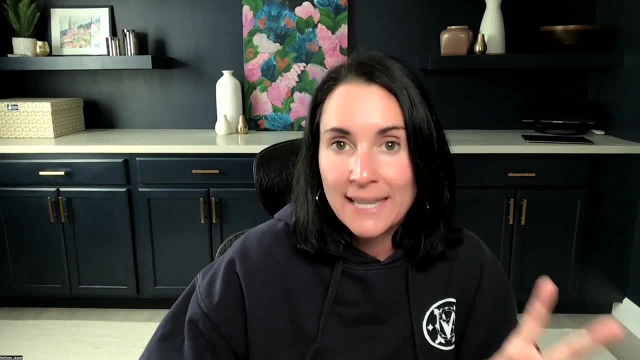 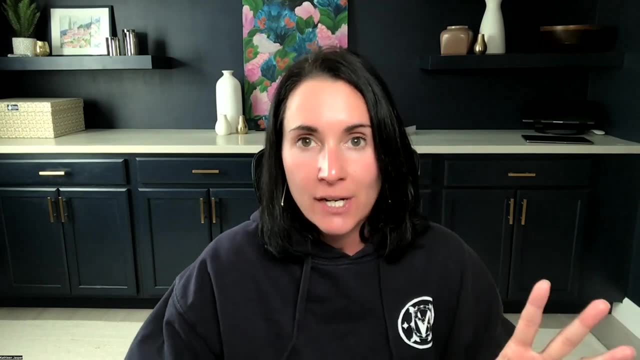 So you can see what you get when you are in the test. it's not very extensive, So you're going to want to really review these formulas as well. So you kind of have them in your head, But if you're stuck on testing you're like: Oh my god, I forget the formula for circumference or I forget the 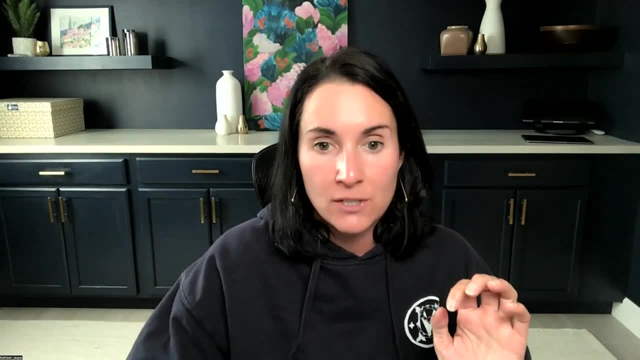 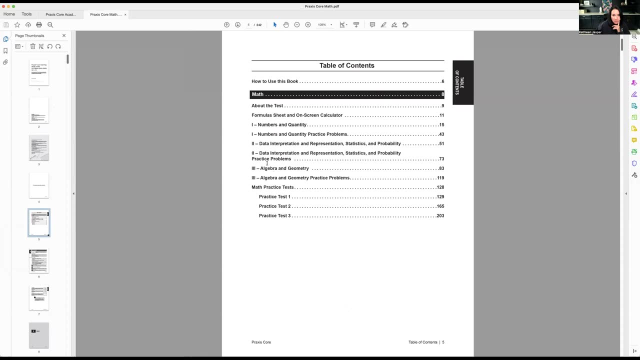 formula for area or whatever. you can find it in the formula sheet. just go to the digital study guide is all linked up. So let's go to the formula sheet and I'm going to go to the formula sheet. go into algebra and geometry. these are the practice problems, But you can see here that we 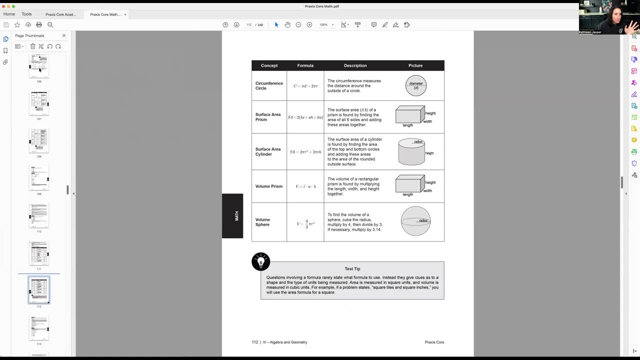 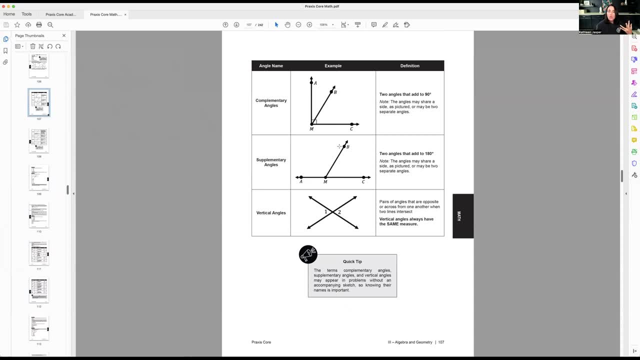 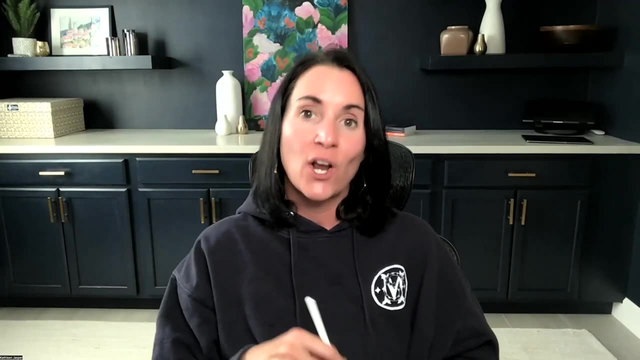 have all of the formulas and the concepts here. let's go to angle measures. Here's what we talked about: vertical angles, supplementary angles, complementary angles. So we provide you with all that information And that's why, when people get the study guide, we stop sharing here. people get 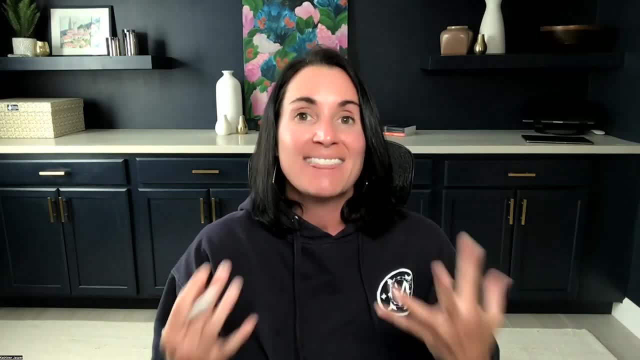 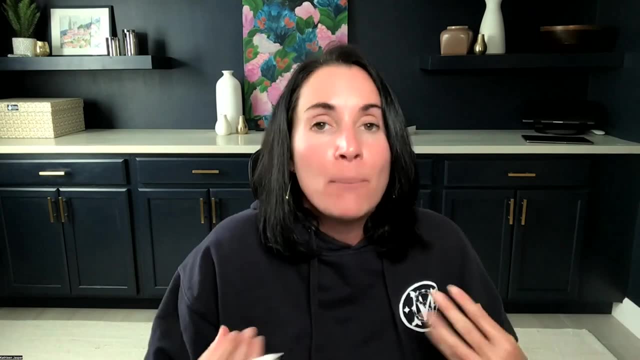 the study guide and they're like: Oh, I just want practice test questions And it's like that's not going to do it, especially if you are lacking in the skills. doing practice tests over and over again is okay, But if you are struggling with the math, you really have to understand those concepts. 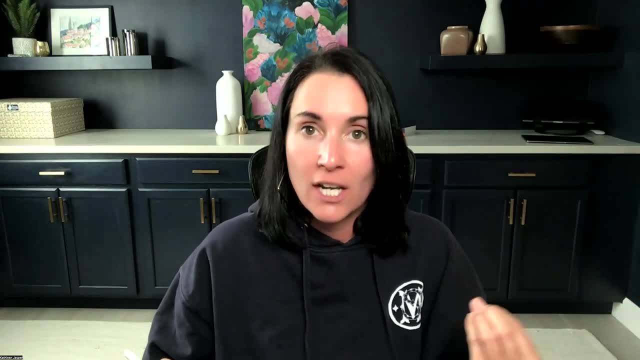 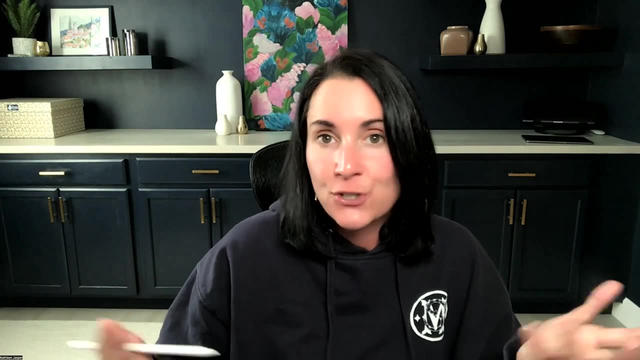 So, going through everything in the study guide- and it's extensive- you're going to need to, you know, do 20 minutes a night, 30 minutes a night for a few weeks, in order to get that information. Now, if you're a math whiz and you were good at it in high school and it's all good, you might. 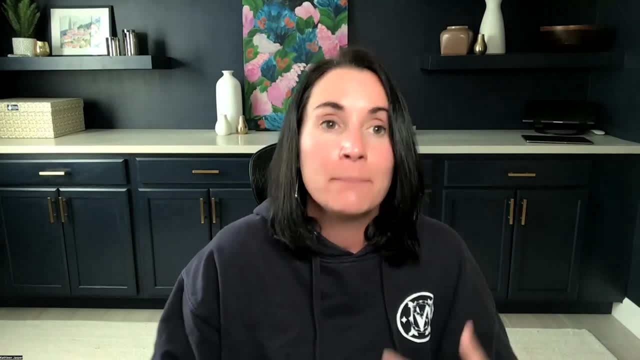 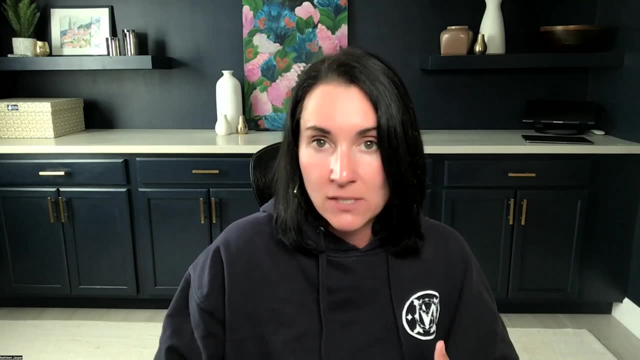 just need a review. If you're someone who struggled with math for a long time, I have tons of videos on this YouTube channel So you can definitely go check that out. And if you're a math whiz, check those out. And we also have an online course for the practice core math. that is very 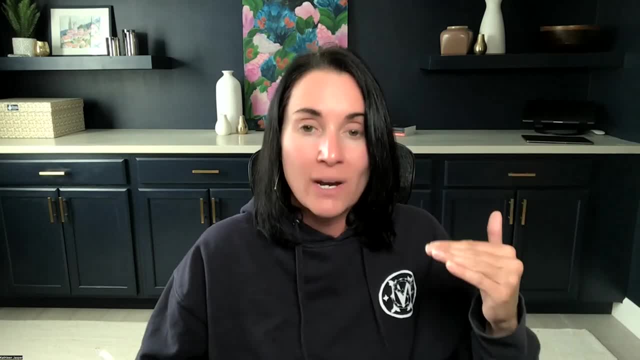 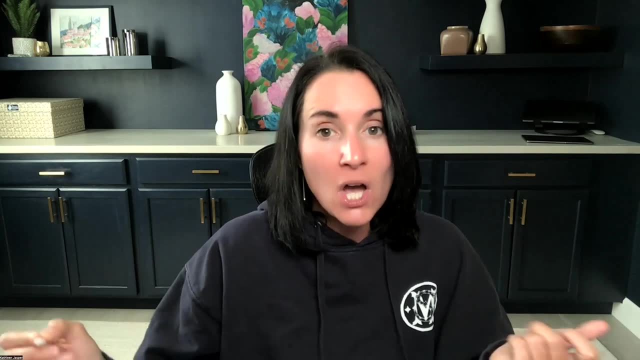 extensive. it has hours and hours of videos. that goes through the book. And then we also have videos for every single practice test question in the study guide. So you can just follow along and work through them, Or you can just work through them, work through the ones that you had problems. 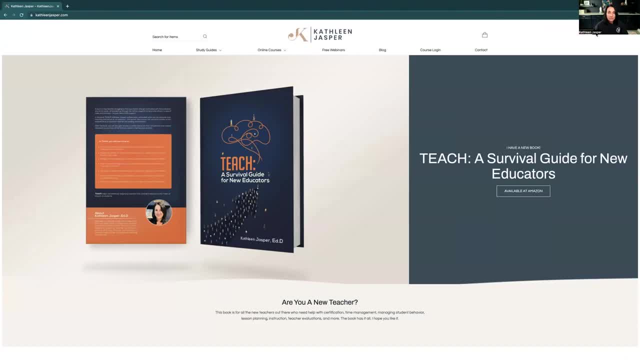 with. Let me show you really quick where to go, And you can find everything we offer here on our website. I just published this new book, teach. you've probably been hearing me talk about it constantly, And I'm going to show you how to do that. So if you're a math whiz, you're going to 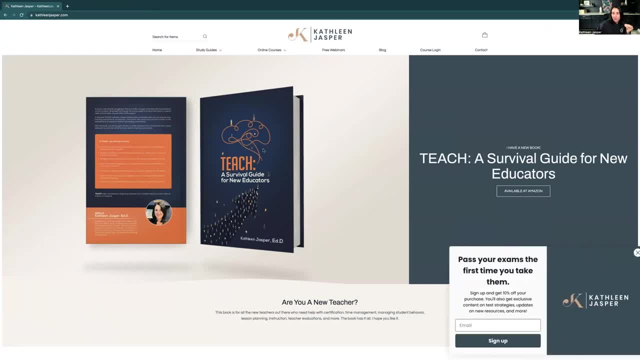 find everything we offer here on our website. I just published this new book, teach. you've probably been hearing me talk about it constantly. This is a survival guide for new educators. This is about the classroom and not necessarily math specific, but there's tons of information here. But if you 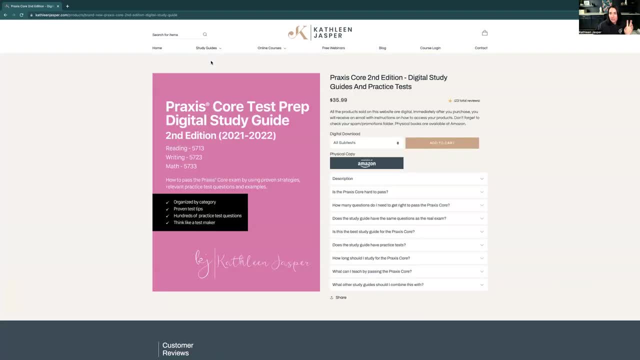 go to study guides. you can see you can get the practice core here And again, I'll link it up in the description below. It's also available on Amazon. you just click this button. it'll take you right there to purchase that. And then, of course, if you are struggling, we have the practice. 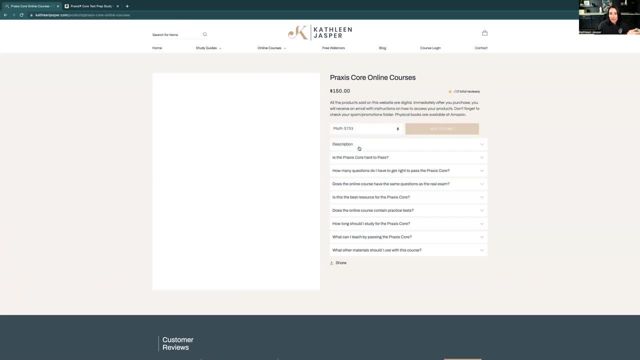 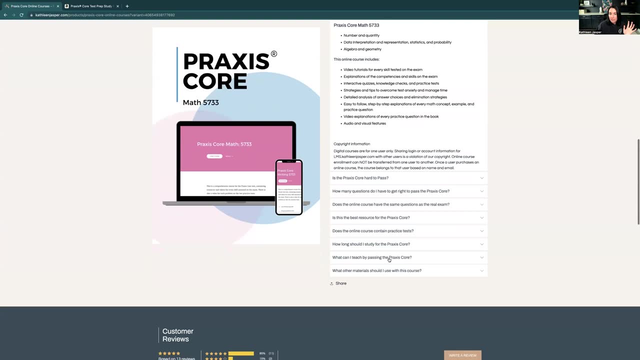 core online course. you can get all of them or you can get the math only you can. you can get them by subtest here And I have a ton of information in these drop downs for you- questions that people ask a lot, So I put them in a frequently asked question kind of drop down box here, And so it. 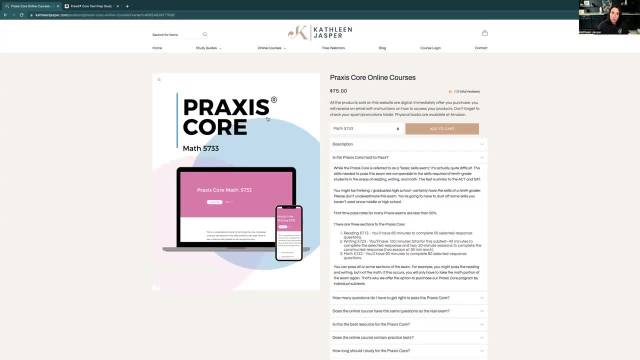 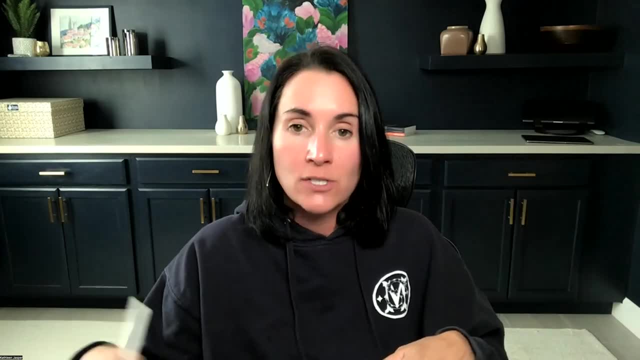 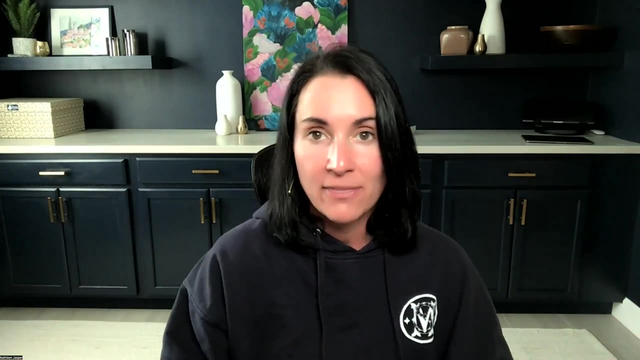 answers all those questions. And again, this is very extensive if you're working on that practice core math. So we got the free stuff on YouTube. we have the practice core webinars. I'll link that up as well. We have the paid stuff: the study guides and the online course. I'm also on TikTok. I'm 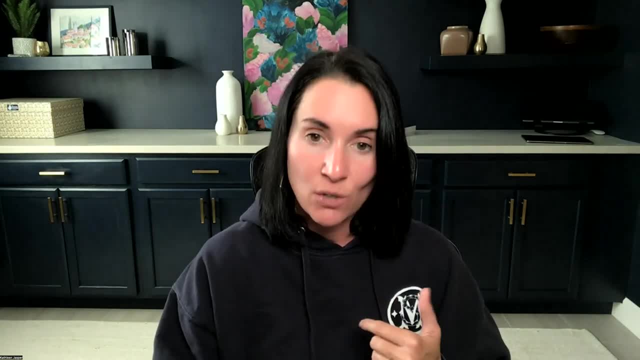 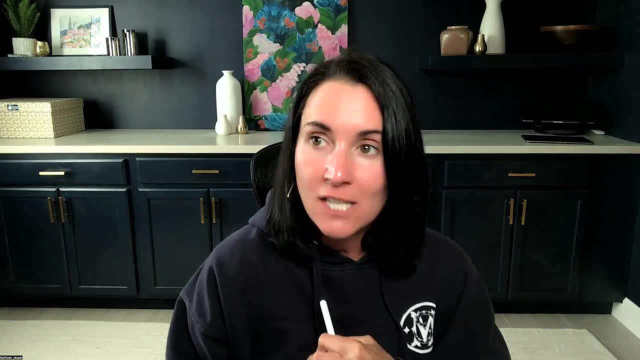 going to post a link in the description below for that We're really amping up our newsletter. I want to provide the best information for you, So if you have any questions, feel free to ask them in the comments below. And. if you have any questions, feel free to ask them in the comments below. And. 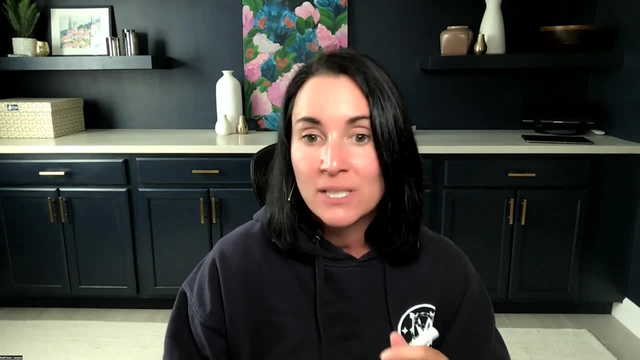 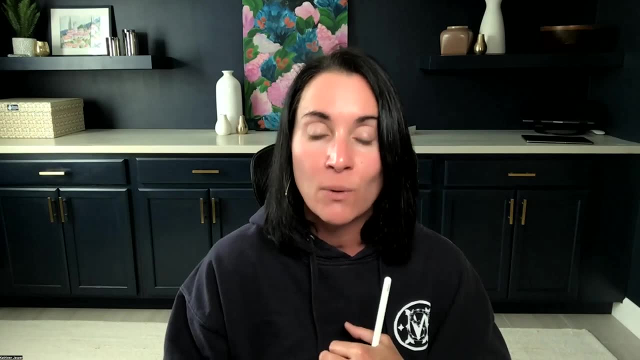 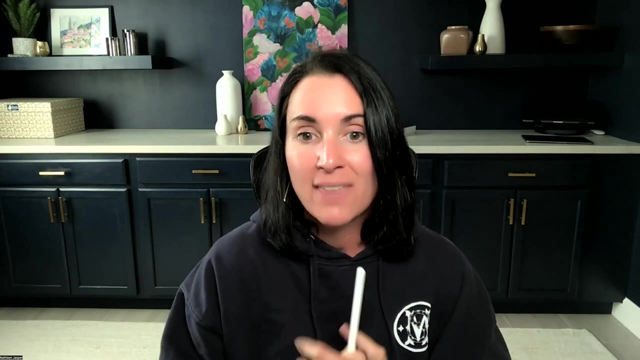 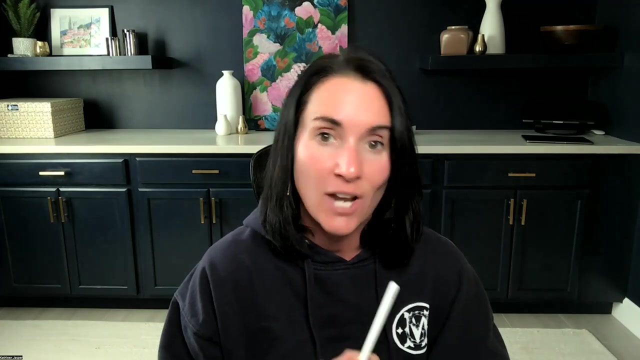 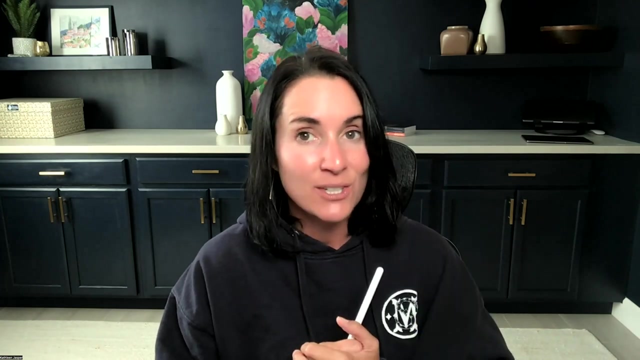 I'll see you in the next video. Take care, take care and I'll see you in the next video. So if you like this, give it a thumbs up, subscribe and I will see you next time. Have an awesome day. Thanks. 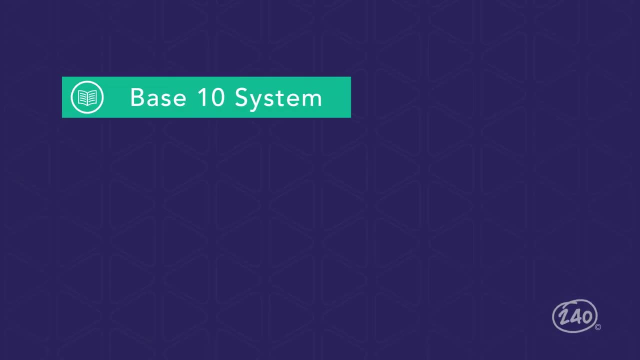 The number system we use today is a base 10 system with Hindu-Arabic origins. A system is base 10 if each place, location for a number has a value, that is, a power of 10.. When a digit is in a specific position, its value is equal to the product of the digit. 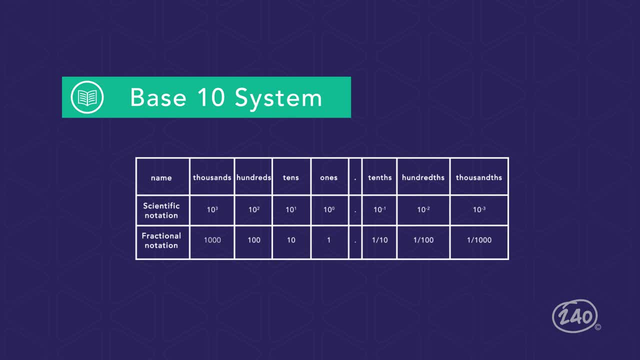 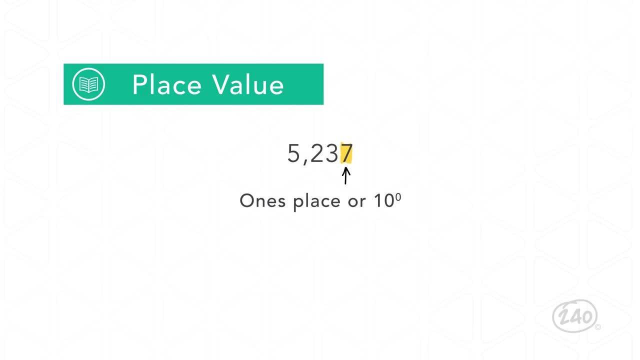 and the power of 10 that is assigned to its position. For example, the 7 in the number 5237 is in the ones place, or the 10 to the zeroth place. It has a value of 7 times 10 to the zeroth. 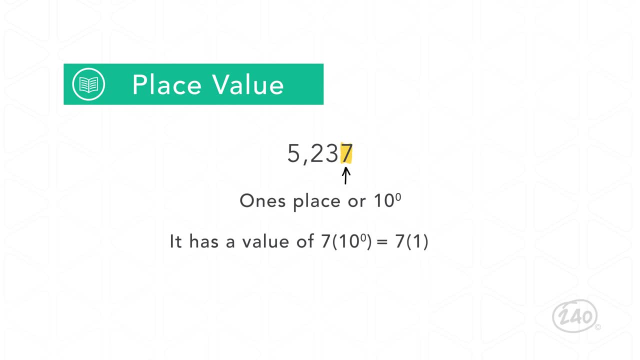 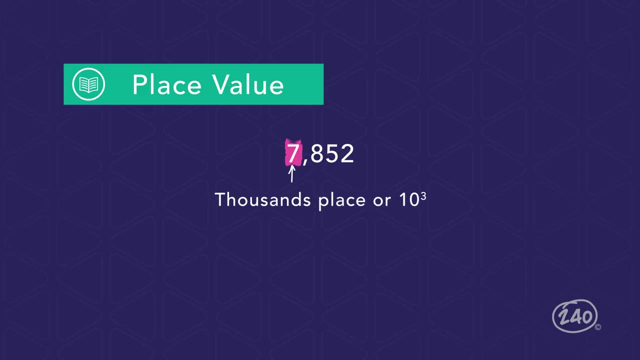 power, which is equal to 7 times 1, which then simplifies to 7.. However, the 7 in the number, 7,852, is in the thousands place, which is also known as the 10. to the third place, It has a value of 7 times 10. to the third power, which is equal to 7 times 1000. 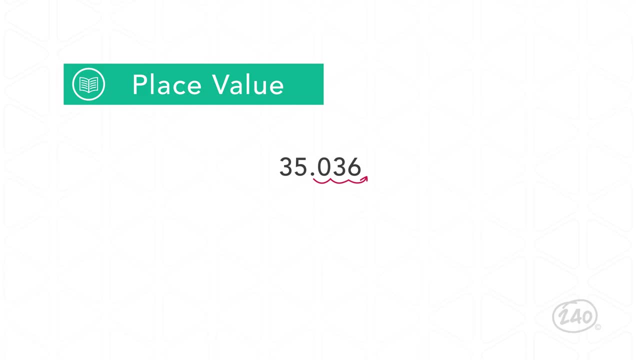 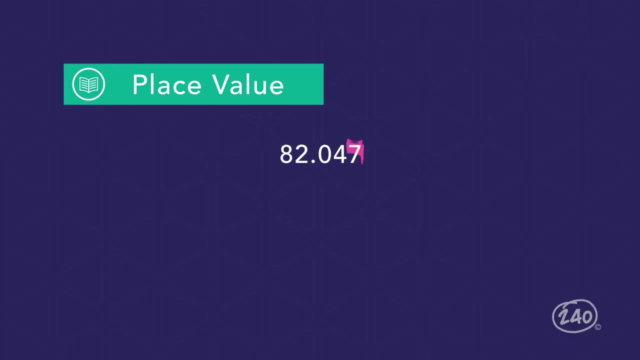 which becomes 7000.. Place values to the right of the decimal point end in THS and have a negative exponent for their power of 10.. For example, the 7 in the number 82047 is in the thousands place, or the 10 to 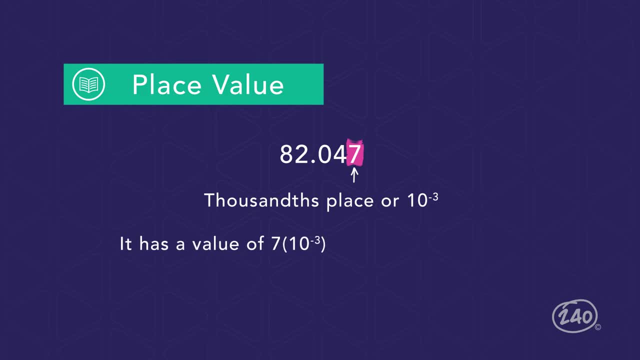 the negative third place, It has a value of 7 times 10 to the negative third, which is equal to 7 times 1, one thousandth. This is equivalent to seven thousandths. Note that in the base 10 system the value zero is used as a placeholder. It represents the absence of a value in a particular. 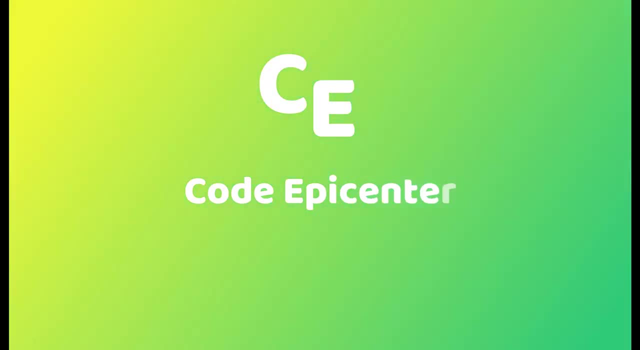 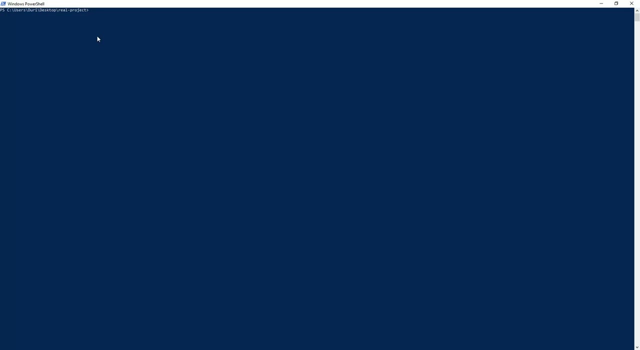 Okay, so welcome back. We are starting with a completely new project, So let's create that project, And we have already learned that. So it's view create and our application is called to do app. So I will just name it like that, And when I hit enter, then here of course.